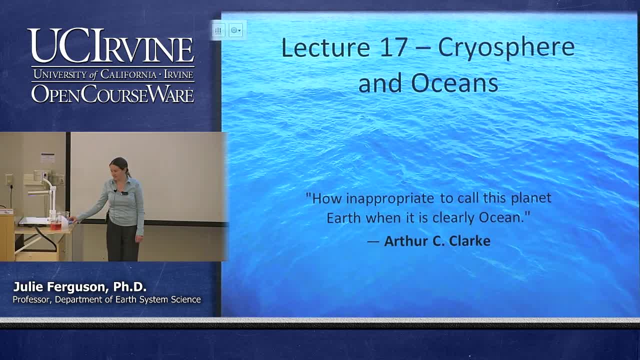 Monday and I managed to not finish my experiment and I'm determined to show you guys that sea ice does funny things to sea level. So I have when I prepared earlier now with a nice line because the pen would work okay, and I've coloured it red a little bit, so you 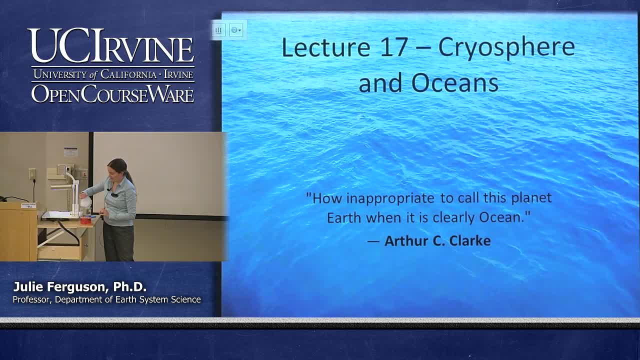 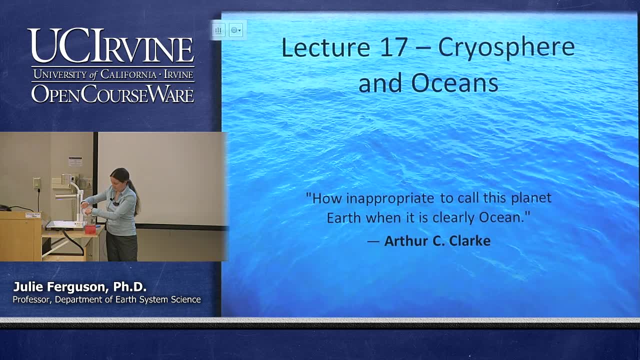 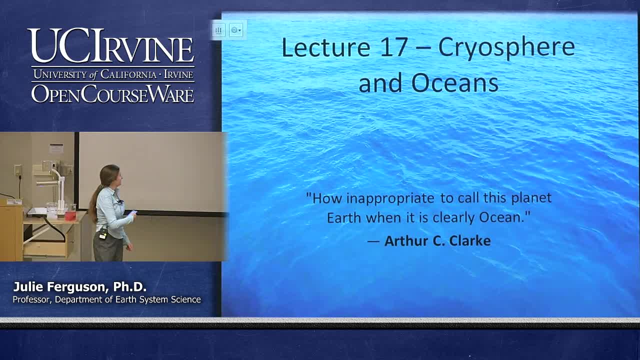 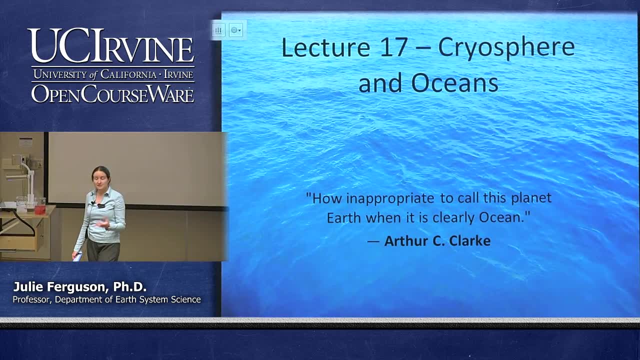 remember to do that and if i don't, someone yell at me, okay so. so we're going to talk a lot today about the oceans, and really the little bit of the cryosphere that we have to cover leads into one of our biggest concerns about the oceans in the next few centuries- well, certainly the next hundred. 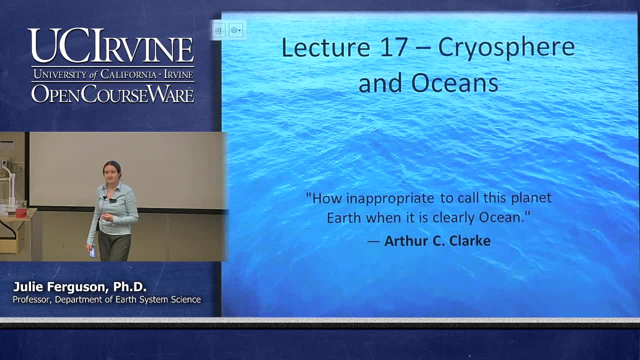 years, but even longer, which is sea level rise, and this is something that, if you haven't heard of, it is an important point. and really, why are we interested in the oceans? because they make up most of the earth's surface. they are enormous. they have very important implications. 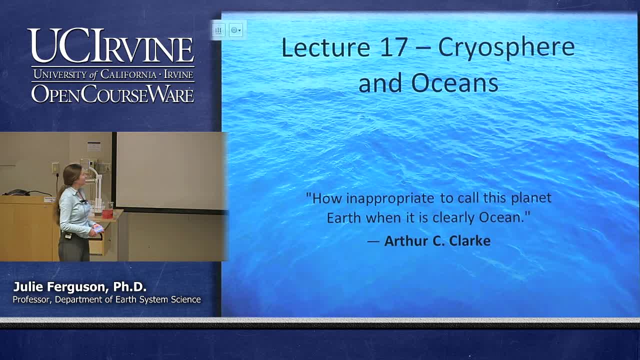 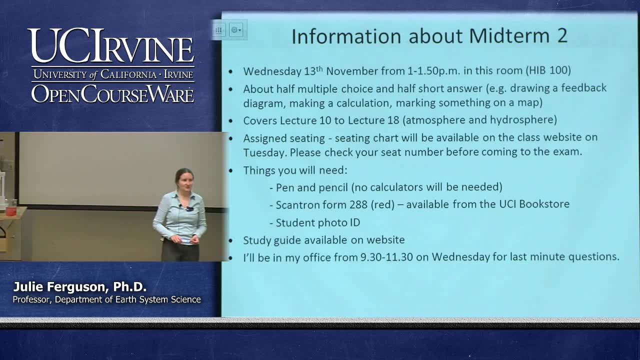 and i love this arthur c clarke quote here, which is how inappropriate to call this planet earth when it is clearly ocean. okay, so i love that little quote, but some bad news. okay, it's that time again. it's gone past quickly, but midterm two is going to be a week today. okay, and it's. 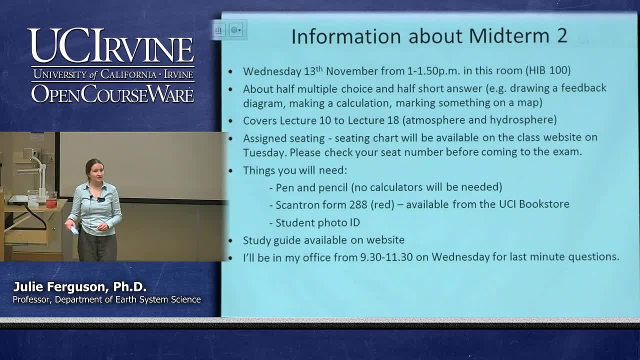 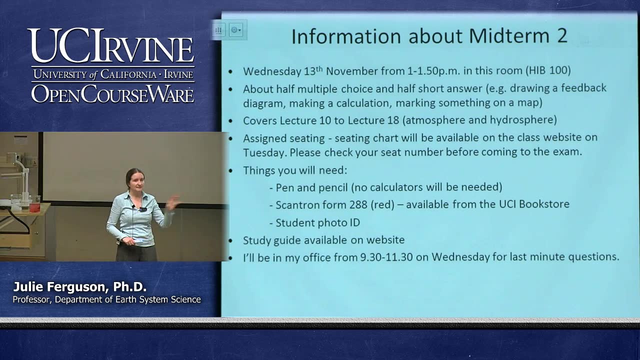 going to cover lectures 10 to 18, so it will include friday's lecture and� And Monday is a holiday, remember. if you didn't remember, So have a look through those atmosphere and hydrosphere lectures. Also, on my study guide, I have a few things that I do expect you to remember from the first little section. 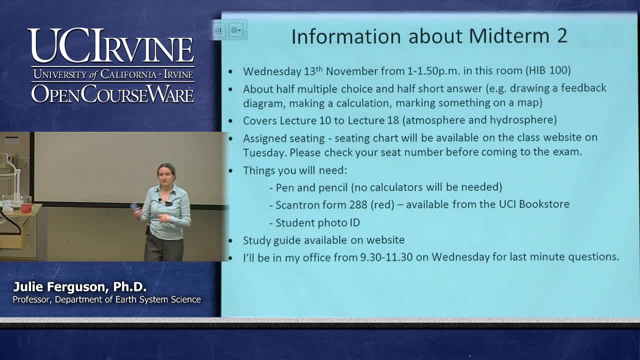 which is just really basic things like energy comes from the sun and conduction versus convection, So those things aren't too challenging to remember. No more sort of pointing out different boundaries. There'll be assigned seating. I have a list of the left-handed people from last time. 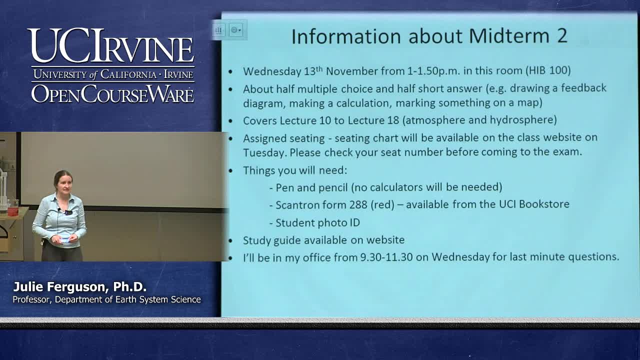 If you didn't manage to email me last time to ask for a left-handed seat, please do this time around, And you'll need exactly the same things. You won't need calculators, The Scantron form, the red 2881, and then you'll have a Part B which you'll fill in on the paper. 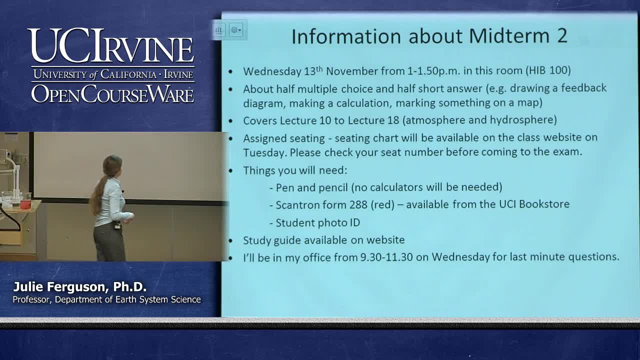 And please do remember your student photo ID. The study guide's already available on the website. In the next couple of days I'll upload some practice Practice questions for Part B along with the answers, okay, So try and have a go at the questions first, and then you can check your answers versus mine. 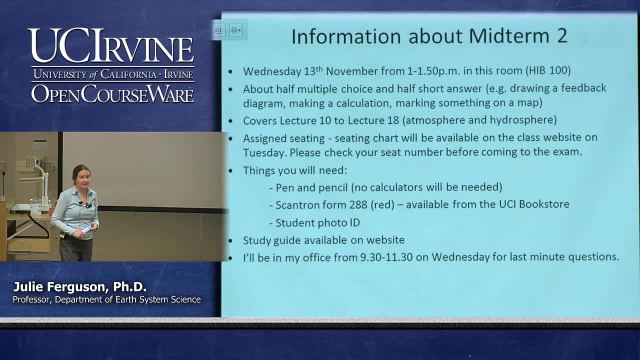 and see if you're following along. okay, And I'll be in my office on Wednesday morning from 9.30 to 11.30.. If you have any last-minute questions, I'd be happy to go over those. So it'll be very much the same as the last time. 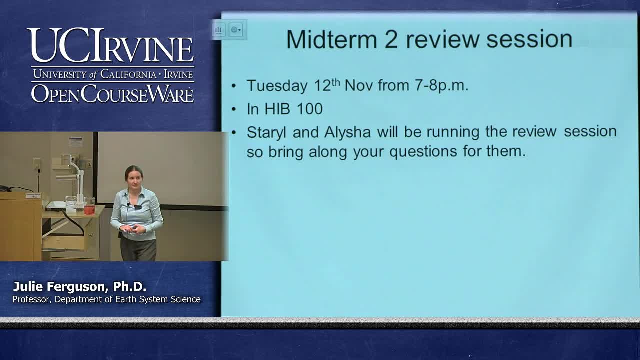 And we do have a review session, so Staril and Alicia will be doing this review session. Okay, And unfortunately, Tuesdays are really busy days. I didn't want to set it on Friday because no one's really studied yet. I know that. 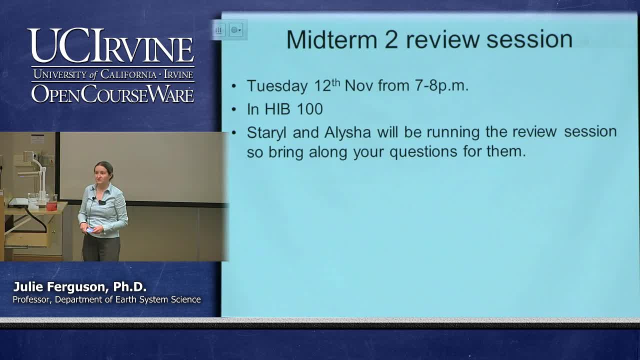 And so Tuesday the only time we could get a room was from 7 until 8 pm, And I know that's really late, so I'm very sorry about that, But it's better than nothing, okay? So bring along your questions and it will be in the same room it was before in HIB 100, along the road. 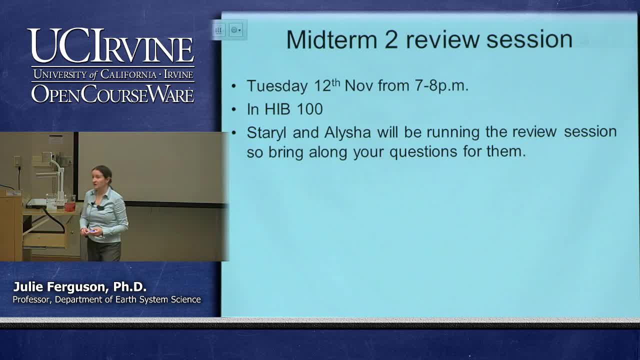 Yeah, Yep, Thank you, I forgot to put that on, But you're allowed to bring one double-sided link Index card, just like last time, so you can bring notes with you. Good question, I'll update that on my slide. 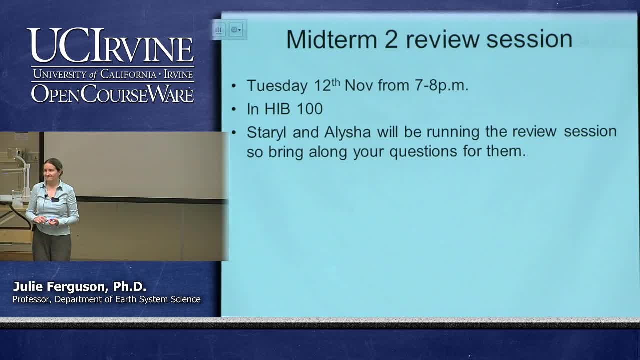 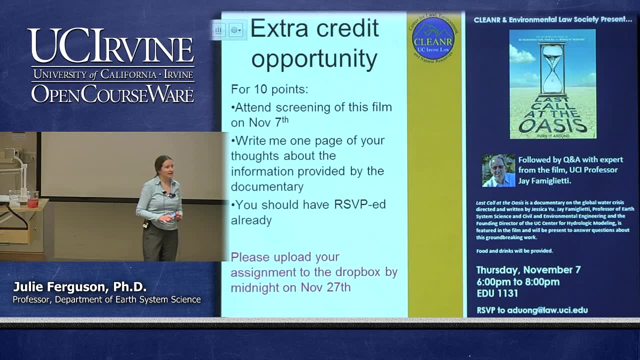 Any questions about Midterm 2?? No, Apart from what will be on it, I'm not going to answer that. Okay, So for those of you who are going on Thursday, did anyone not manage to get a seat? who wanted to go? 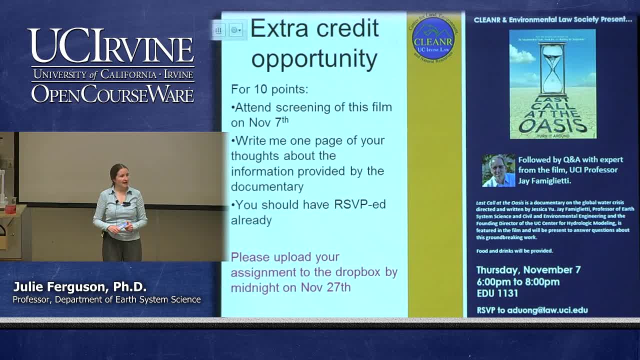 Oh, really A few of you. Okay, I have a copy of the DVD. Perhaps you guys could watch it in groups Or something, if you are still keen to do so. It is also available online, So you might be able to find it online. 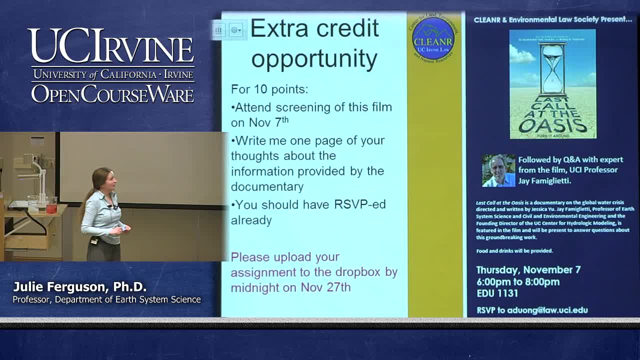 Let me know if you've had problems with that, Okay, So I do want to mention the deadline for this, though, which is November 27th. That will give me a chance to grade it over Thanksgiving weekend, okay, So if you're going to attend, really if you're going to be writing reflections on it, 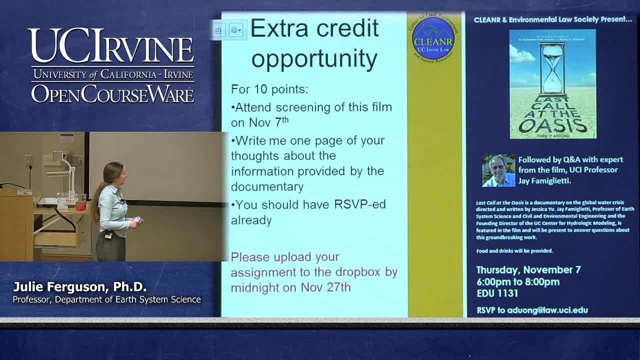 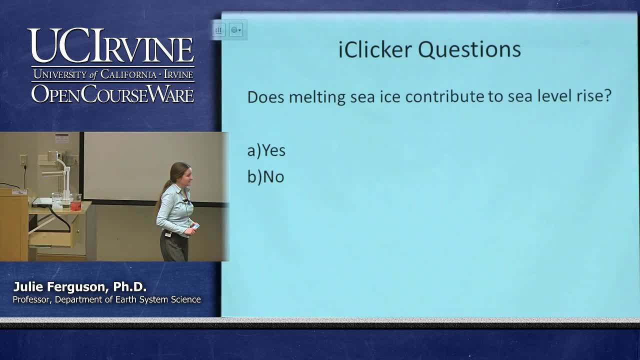 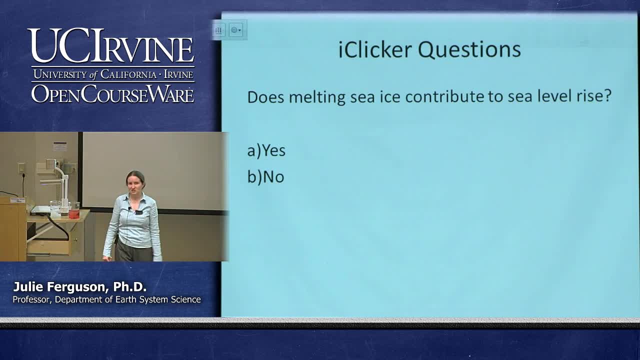 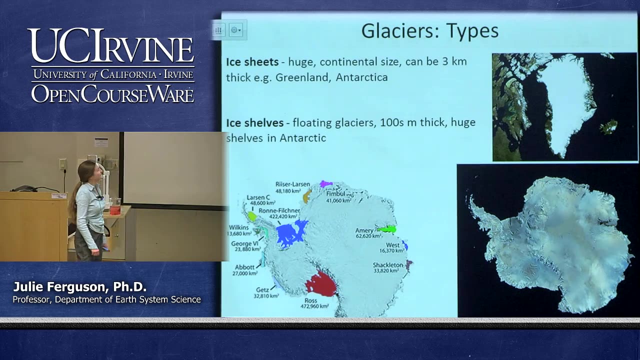 70% of people said yes. 37% of people said no. Okay, So I'm actually going to ask you this question at the end, when you can actually see what's happened. Okay, So let's move swiftly on to So. we talked about the smaller versions that we get on land. 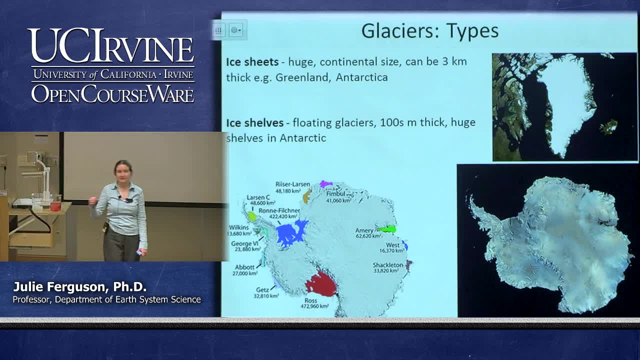 We talked about little cirque glaciers, valley glaciers, the fjord glaciers- where they meet the ocean, and ice caps, which are these larger areas of ice, but really by far the most ice on the planet is in Greenland and Antarctica are big ice sheets okay. 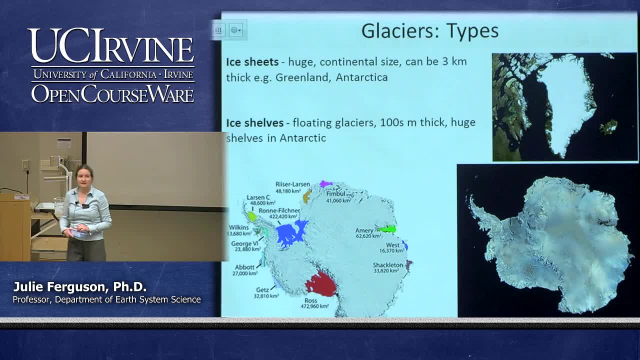 And associated with the ice around Antarctica specifically, and we have what we call ice shelves. Okay, So ice shelves are floating areas of ice again, so they're floating on the ocean, although they originally formed on land. so they're different from sea ice. 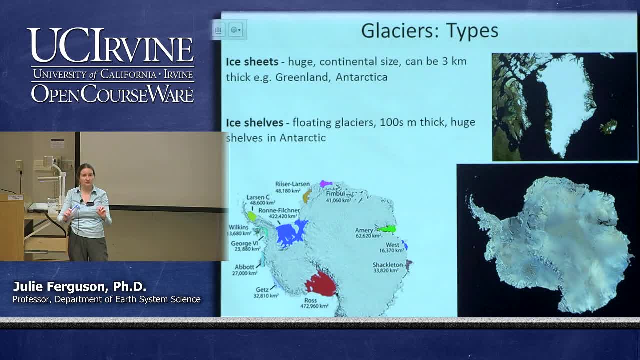 Sea ice is what happens when you cool down seawater enough and it just freezes along the top. Ice shelves are when big areas of ice spill off onto the ocean and extend outwards. okay, And those little colorful areas represent ice shelves, okay. 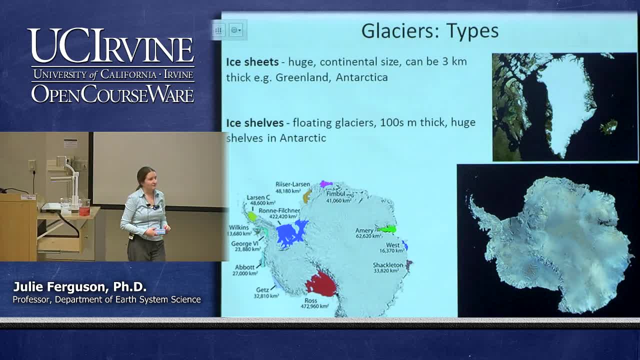 And you can see that we have Larsen's Sea And we use that And we used to have Larsen A and Larsen B but we've lost those And there is concern that these ice shelves breaking apart is sort of an early sign that. 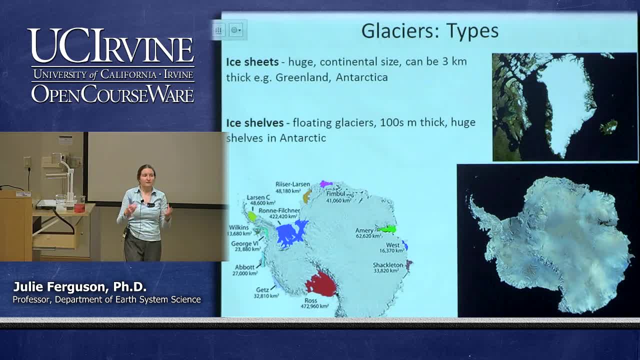 the edges of the continent especially, are warming, And so the floating ice doesn't necessarily contribute to sea level, but those ice shelves act to hold back the ice trying to come off the land. okay, So if you have a nice ice shelf, it slows down the glaciers as they approach the coast. 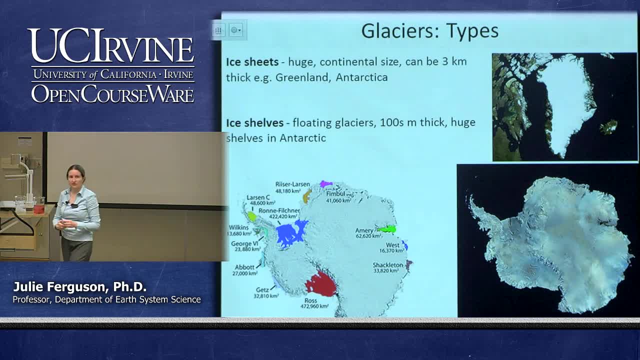 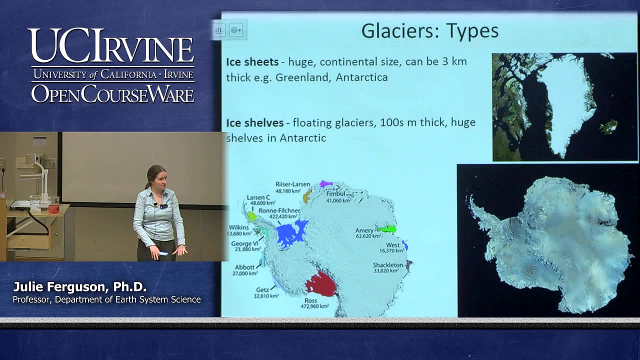 okay, Okay, And it slows down the ice that's going into the ocean, which does raise our sea level. okay, And our ice sheets can be 3 kilometers thick. Think about what that is: 3 kilometers thick. That's so heavy that it's actually weighing down the continent, the whole of the Antarctic. 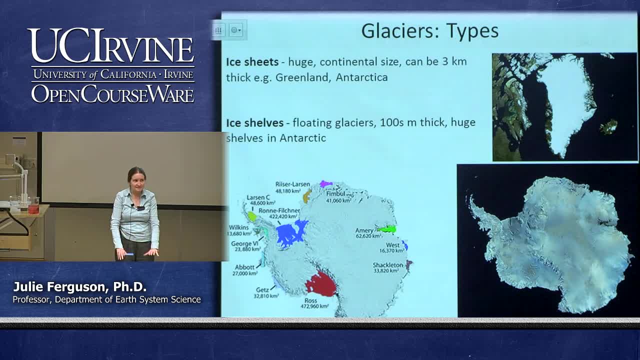 continent. Most of it is below sea level because it's being weighed down by these ice sheets, And the same is true of the center of Greenland. If all of the ice melted on Greenland, actually it would be below sea level, would be below sea level in the middle because of the weight pushing down, just like if you pile. 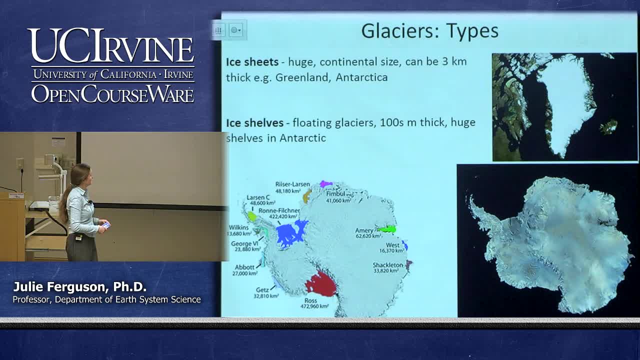 more people onto a boat or one of those floaty things. they sink, okay. and our ice shelves- these aren't little sort of meter thick, sort of sea ice. these are hundreds and hundreds of meters thick. you can park one of the giant us sort of boats next to it and they start to climb up to get on. 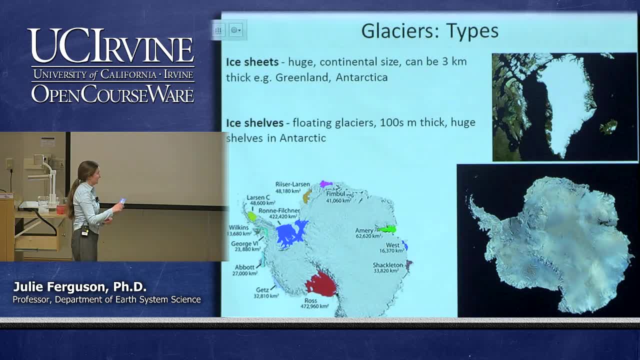 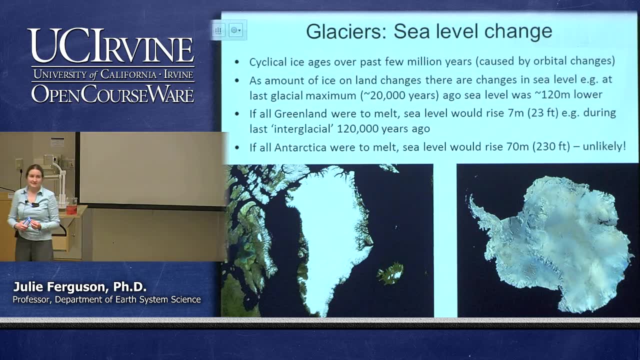 top. okay, these are really big pieces of ice and they're amazing. if you ever get a chance to go see them, do go. but why are we concerned about it? we're not concerned necessarily because people live around there on greenland. there's people around the edges but very few people. the reason: 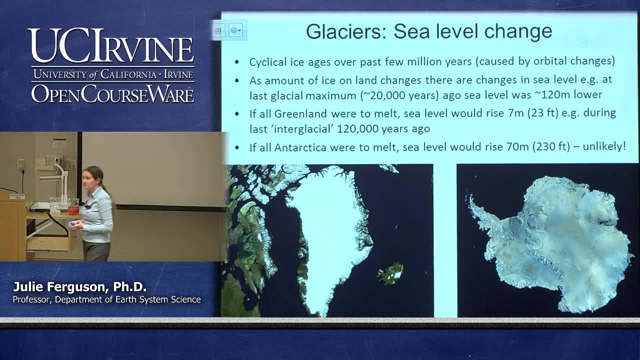 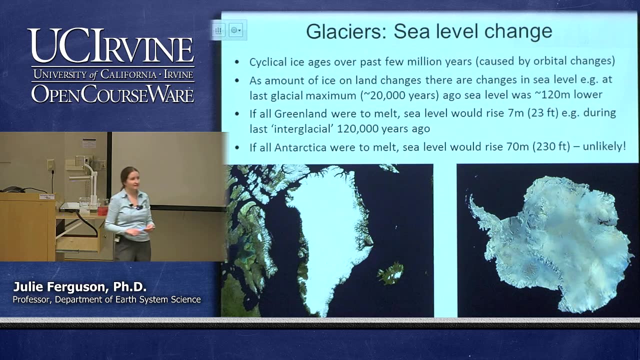 that we're concerned about changes in these is first of all, albedo again, but much more selfishly for us, it's sea level. if we melted the whole of greenland, our sea level would rise by seven meters, and i've put it there in feet as well: 23 feet, okay.